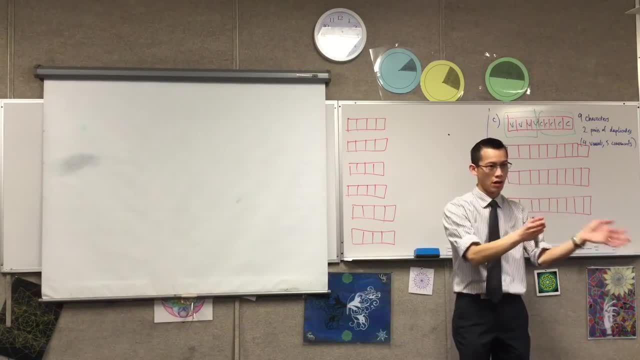 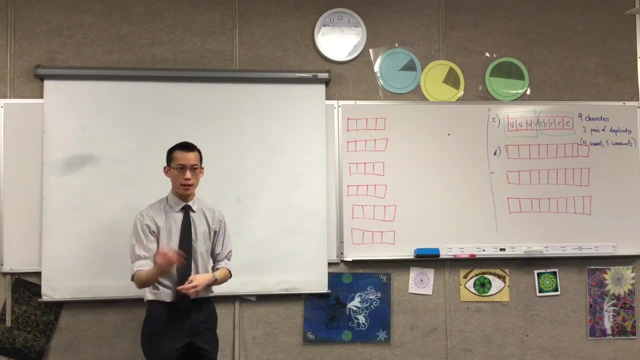 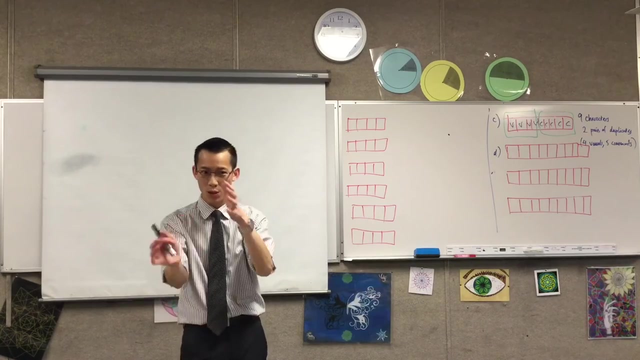 That's one of the great things about mathematics: No matter which path you go, you should arrive. if you've used an accurate method, you should arrive at the same conclusion. So I'm going to show you three ways. These are all sort of principles. They're not about like: oh okay, this is a set of steps that I can memorize, because you'll get a different question and it will ask you a slightly different thing. 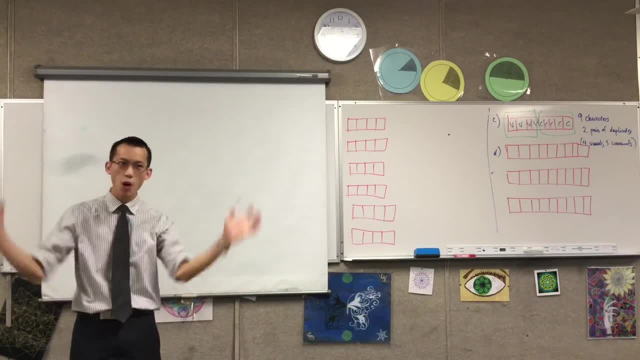 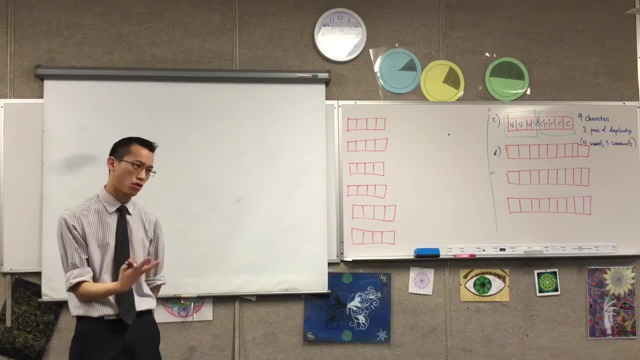 These strategies will work with this particular question, but sort of take the overall principles as much as you can. I'll refer to them in a second. So here comes approach number one, And I think this is probably the most common one, which is why I'm doing it first And I'm calling this. you might want to label this. approach number one is by cases. 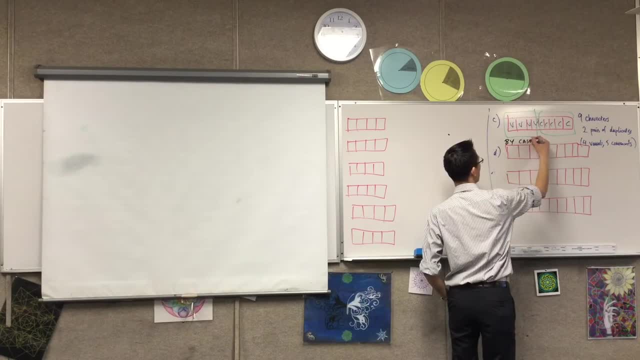 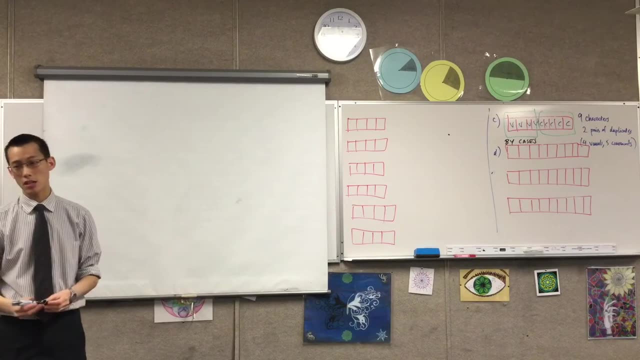 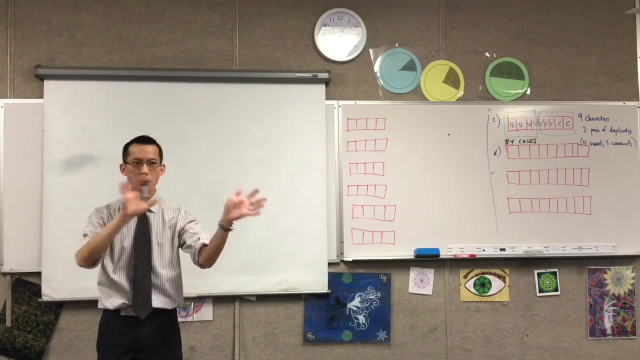 By cases. Now I've got to try and break down this question, And what makes it challenging in the beginning is that what have we got? I think n is supposed to be to the right of d right, But you don't know where either of them are, And so it's like, well, I can't say, oh, there are only eight spots. 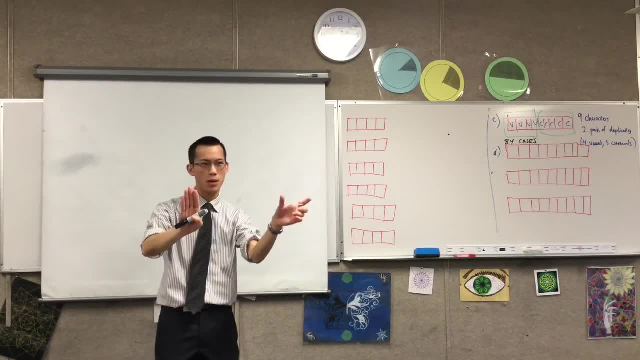 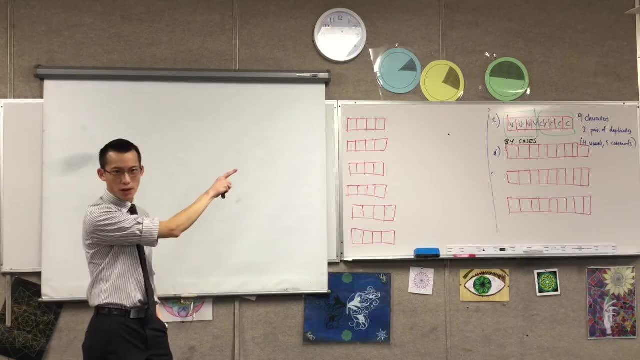 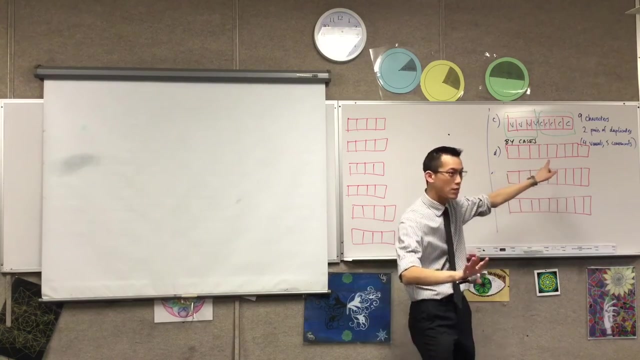 For n because, depending on where d is, it's like: well, there might not be eight spots, There might be only one spot for n And d can move anywhere it likes right, But it can only move in nine spots. Do you see that There are only nine spots for it to sit? So what I'm going to do is I'm going to try and think about each of the cases for where d will be. 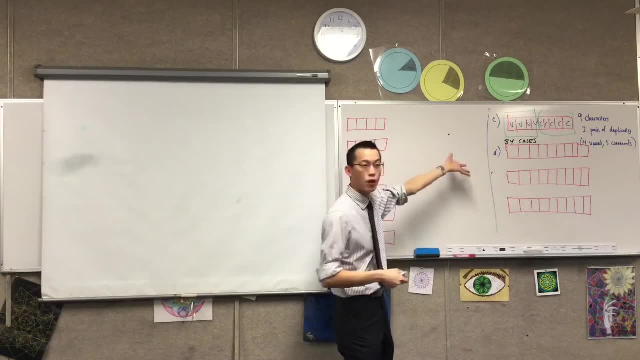 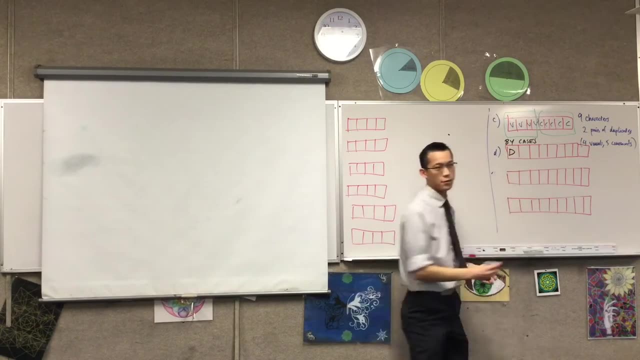 I'm not going to do all of them, because I should be able to get a pattern. You can see I've got three, because three is my standard way of establishing a pattern. So let's think about it nice and easy. I'm going to start with the left right. 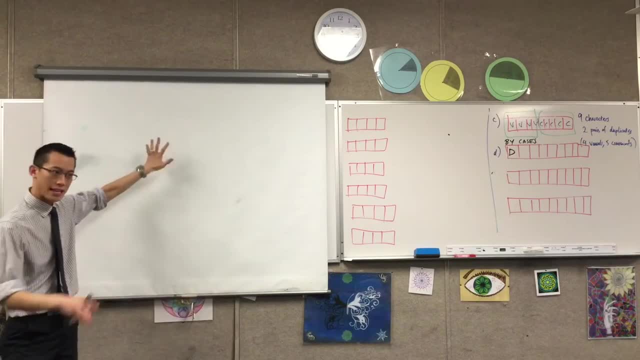 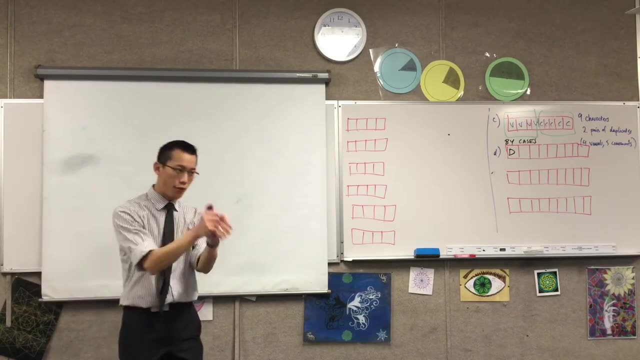 So the way I would work this and I actually would write this, I'll show you at the end of this. I'll show you the way I've written up my full solutions, rather than the way I've talked through it. But I would actually say, next to this diagram, I would say: fix the letter d in position one. That's what I would actually say, right. 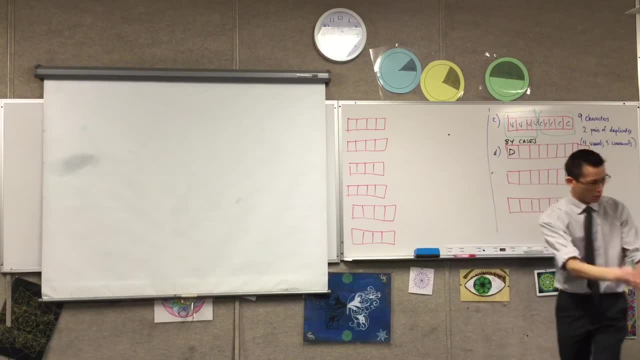 Now, once you've done that, we deal with the restrictions, one at a time. okay, The other restriction is on n right. So where can n be? How many places can it be? It can be anywhere, in any of these spots. 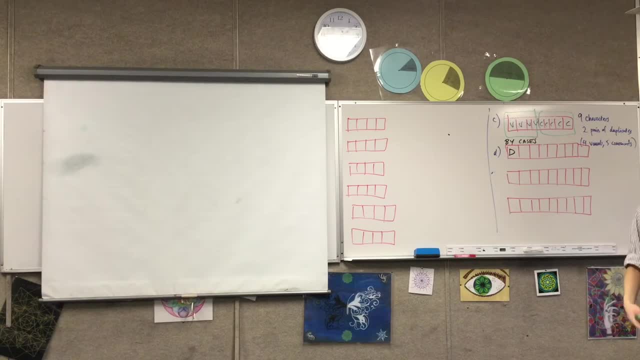 Right? So since it can be in any of them, I actually can consider n as one of the regular letters, right? So what I've got is being that n can be anywhere, right? therefore, it's like: well, I've just got eight letters that I can place in any way I like, right? 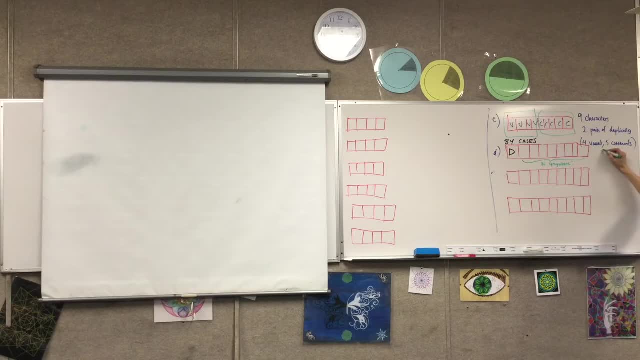 So the way to arrange eight letters is a factorial, but don't forget, I do have repeats. What I'm going to do, is you notice, I'll have repeats every time I do this, So I'm going to worry about the repeats right at the end. 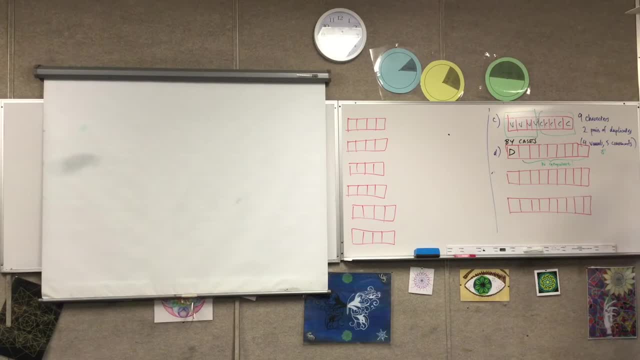 Let's just think about eight letters. okay, So that's fine. Okay, so I've got that. The next case. this was the first case. The next case is: well, let's just shuffle d over. Let's just shuffle it over, like that. 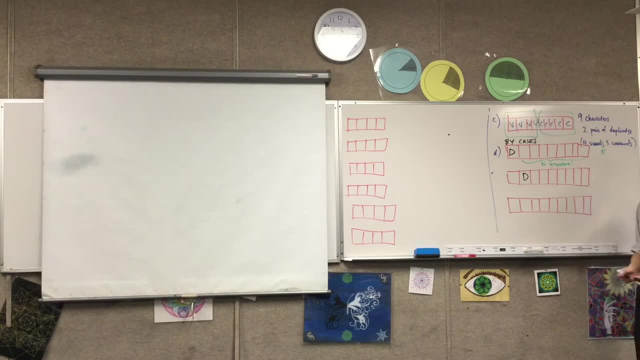 Okay. So then again I ask the question: where can n be? And this time it's a little trickier, right? How many spots have I got left? How many spots can n occupy? okay, Any of these spots, of which there are seven, right? 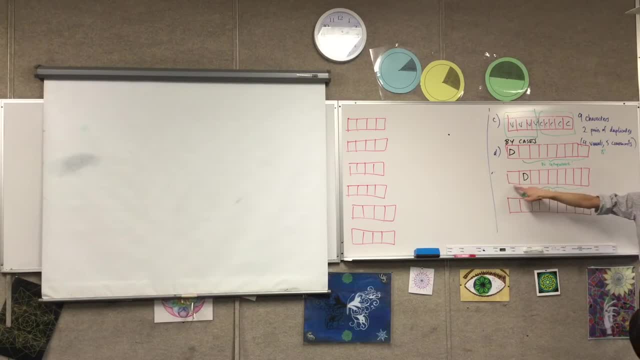 These two are taken. Well, this is taken and this one doesn't fit our conditions, So therefore, I've got seven left. okay, So there are seven ways to place n. right. After you've placed n, how many letters do you have left to place? 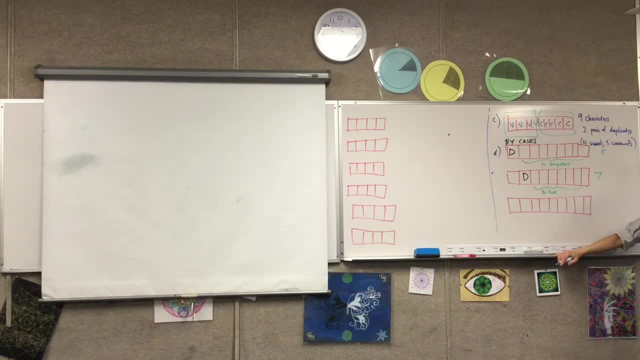 You've got. you've placed d. you've placed n. you've got nine letters in total. So there are seven left to place in all of the other spots. Are there any restrictions on the other letters? No, They can go anywhere they like. 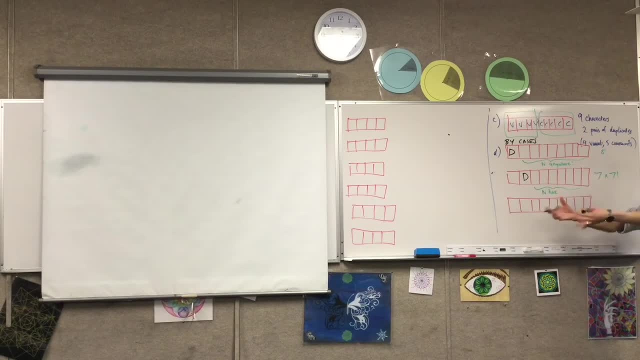 So there are seven factorial ways of placing. They're placing the final letters, the remaining letters, Does that make sense? Wait so one second. Why did you say eight factorial before? Yeah, And why did we say eight factorial times seven? 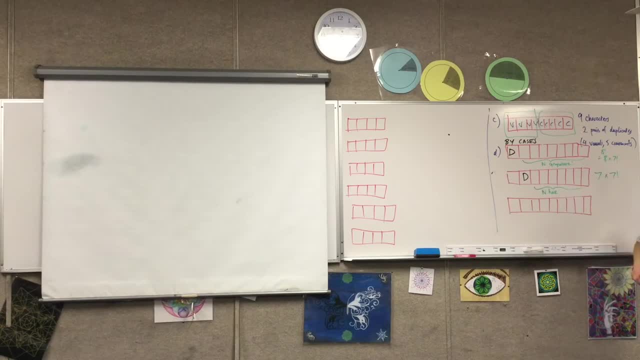 That's a great. that's a great question. I will point out that this is the case right? Think back to how I arrived. and this is pause on this. Take your time, Don't rush through it. You must ask these questions. 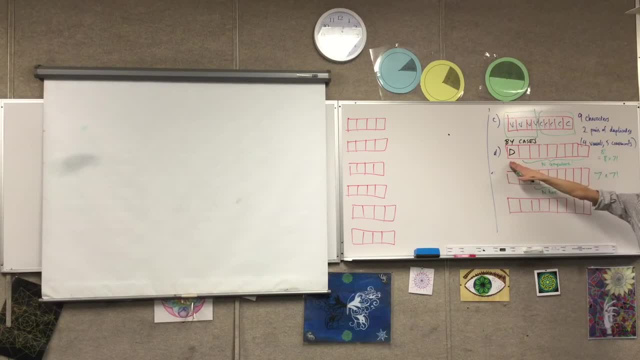 Why did I say eight factorial? Because I placed the first letter and then I realized you know what Eight can be anywhere There are. you know, like I've looked at this is the number of spots that go, but n can be any of those. 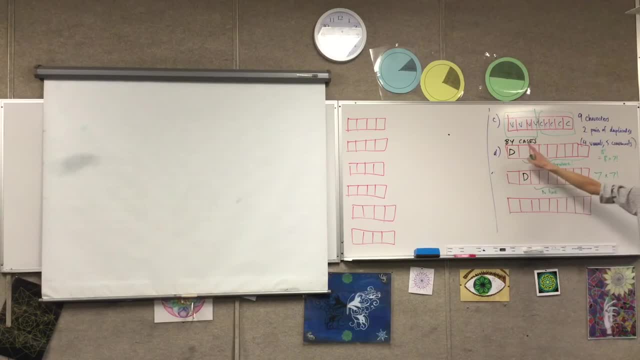 So since n is just one of the regular eight letters, it's just. this problem becomes. this first case just becomes: put eight letters somewhere And that's eight factorial right, And I'll worry about the repeats afterwards, okay, Another way of thinking about it is just like I thought here. 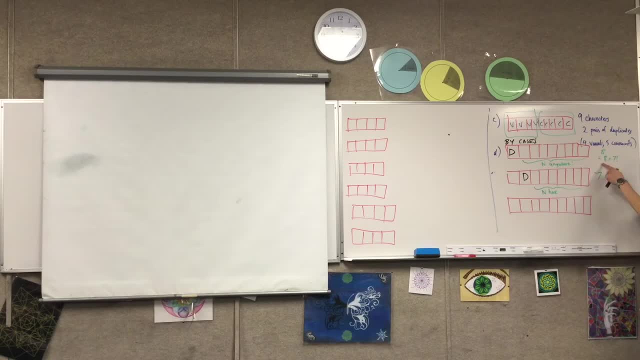 how, where can, where can n be, And the answer is in eight spots. And then I have seven random letters that I don't care where they go. Eight can go in seven factorial ways. Does that make sense? Okay, And this will be helpful because it'll help me establish my pattern. 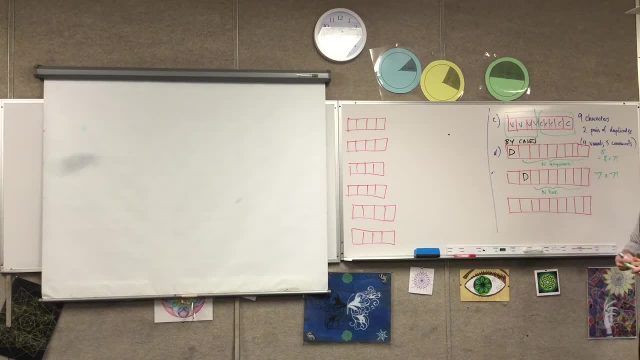 Okay, I've done case one. I've done case two, Case three: Where's d going to go? So the way I would write this is I would say: fix the letter d in position three. Okay, Where can n go now? 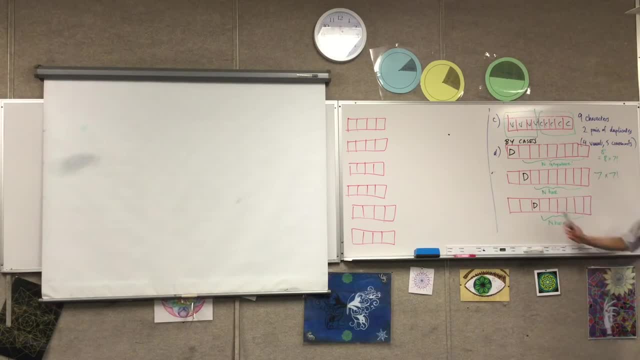 There are six spots left for n right, Because this one's taken and these two are duds. So I will say: here we go. there are six ways to place n, And then I've got seven more letters, right. 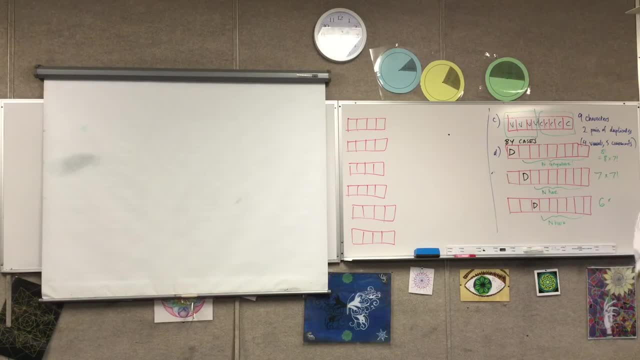 That I have to place. Are there any restrictions on where they go? No, So there are seven factorial ways to place the remaining letters, right? Do I have enough of a pattern yet You can see what's going to happen, right. 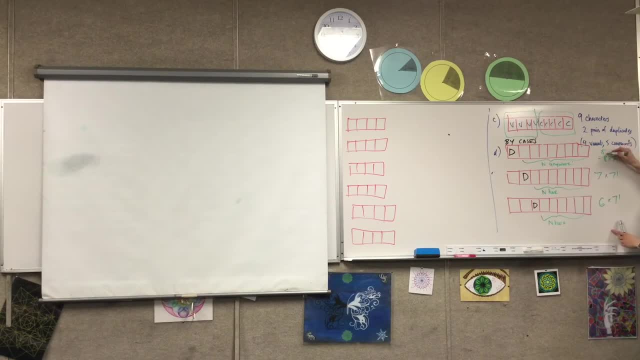 Every time d shuffles over, it's making this number smaller because n gets crowded out gradually. okay, Now remember, I said to you: n can be sorry, d can be in nine spots total, right, Because there are actually nine spots, right. 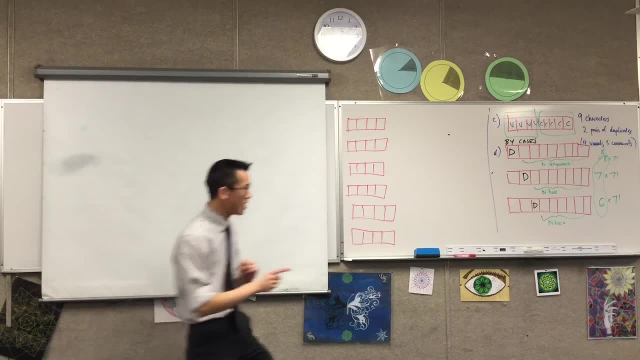 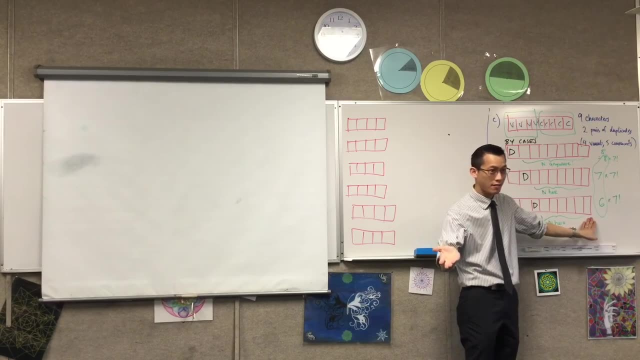 But it can't actually be right, Because if it went over all the way to the end, right, d is over here. how many spots are there for n? There are zero. So in fact I can consider as a case the ninth case right. 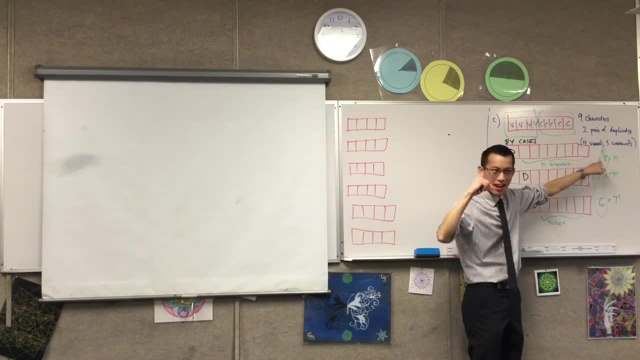 But see how I started with eight. If I'm counting down nine times, the last one will be zero spots for n, and then you place your other letters. but it doesn't matter, because there are no ways that fit your conditions, okay. 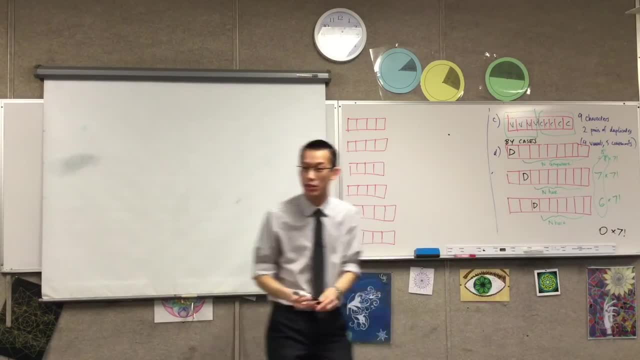 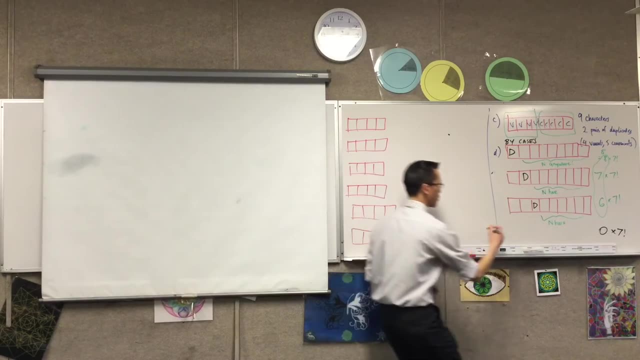 But I'm not going to worry about that. I'm not going to worry about that because it doesn't add to my total. Okay, so now that I've done three cases, I think I've established the pattern. So therefore, the total ways are. so I have a look. 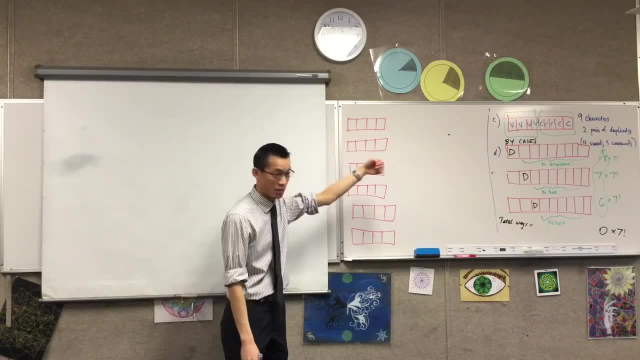 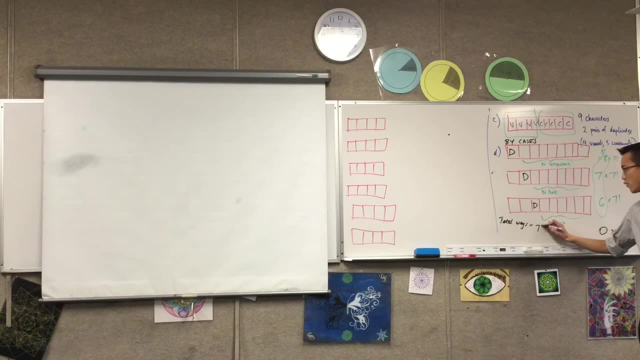 The first one case, one eight times seven factorial. Second, one seven times seven factorial, and then six All the way down. it does go down to zero, right? So I'm going to say there's a seven factorial every time.